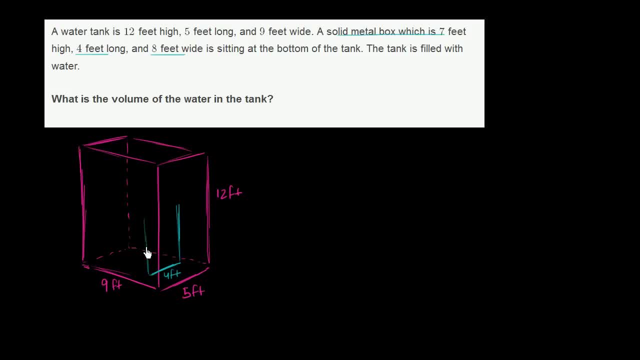 It's 7 feet high, which might look something like that: 7 feet high. Obviously, I'm not drawing it perfectly to scale 7 feet high and 8 feet wide, So it might look something like this as it's sitting in this tank. 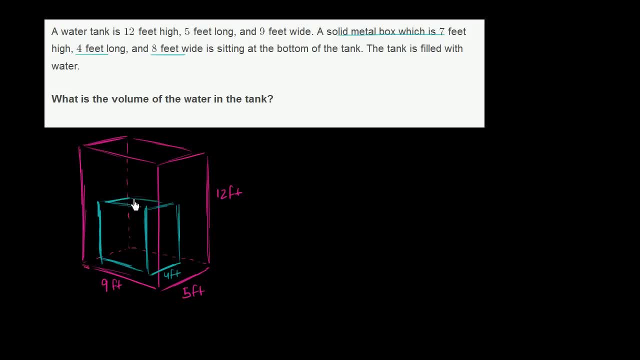 So this is that metal box And they say it's a solid metal box. It's not like any water can fit in here, So let me make it as a solid metal box. So this is a solid metal box, And then I'm going to fill it. 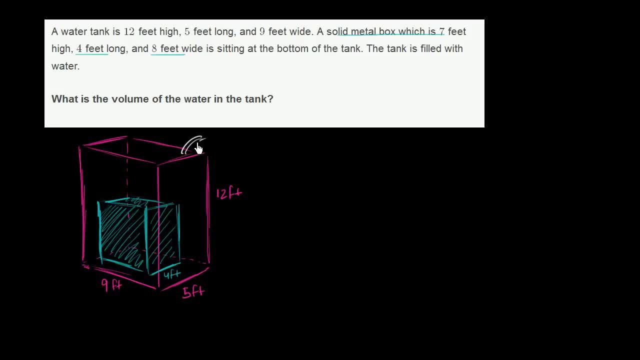 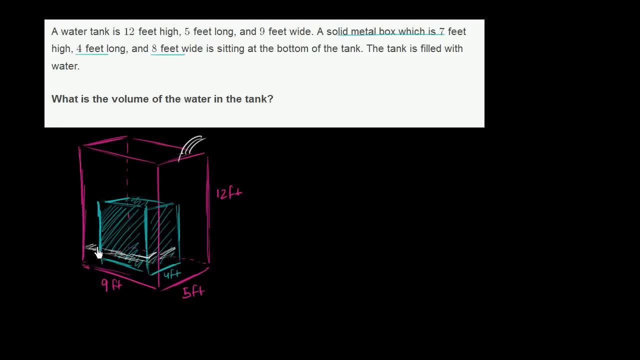 except where the metal box is. It's not going to be able to fill in that volume because the metal box is solid. So it's going to fill up. We're going to slowly fill this thing up around the metal box. So what's the volume that it's going to fill up? 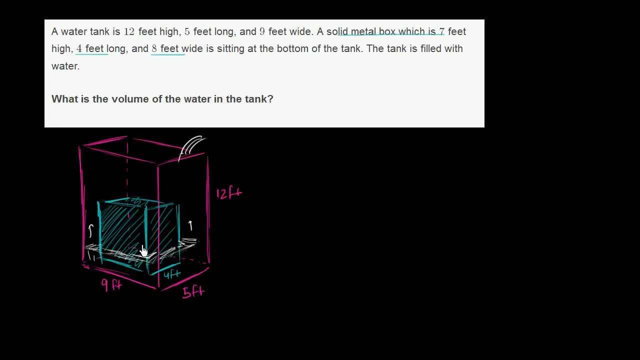 Well, it's going to fill up the volume of the tank minus the volume of the metal box. It couldn't fill in the metal box volume, So let's figure out what that is. The volume of the tank is going to be 9 foot by 5 foot times 12 feet. 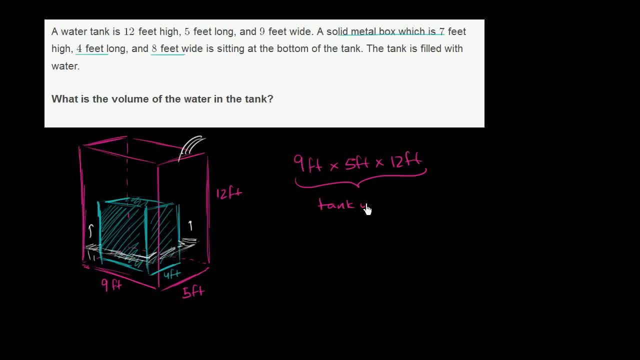 That's the volume of the tank, Tank volume And from that we want to subtract the metal box volume. So minus 4 foot by 8 feet by 7 feet, This is 4 feet wide. It is 7 feet high. 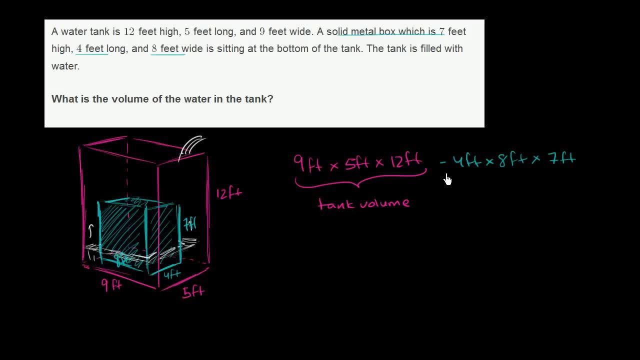 It's 4 feet long And it's 8 feet wide. So this right over here is the volume, This is the- I guess we could call it the metal box volume. And so what's in between? or when you take the tank volume, subtract out the box volume. 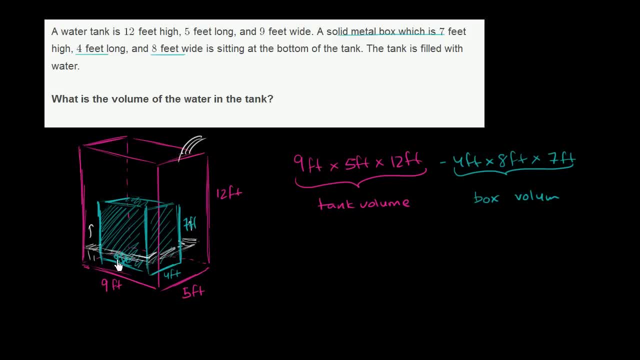 that's how much the water can actually fill in. So I only do the water partially Fill in. But once it's already filled in, the water is going to go all the way to the top here And it will fill in everything, except for where.